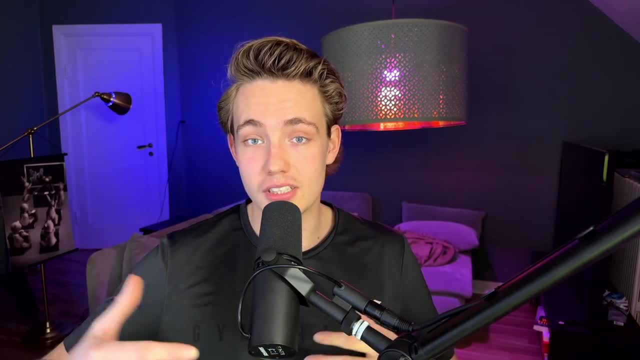 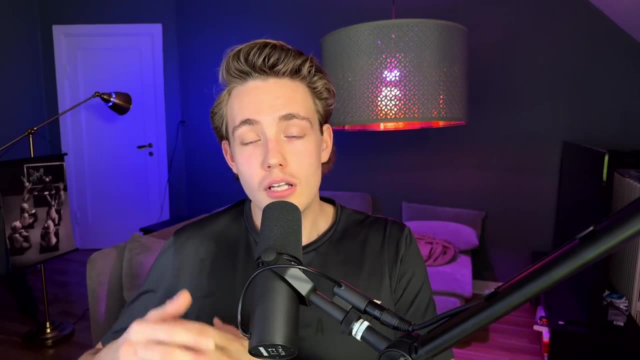 really low fundamental level so you'll get like the basic understanding. The tutorials I have here on the channel about computer vision is basically going from like the beginner level to more intermediate level and then at the end here we act like at a pretty high level where we're combining. 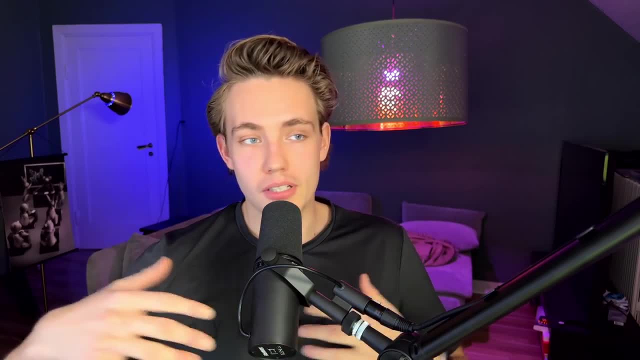 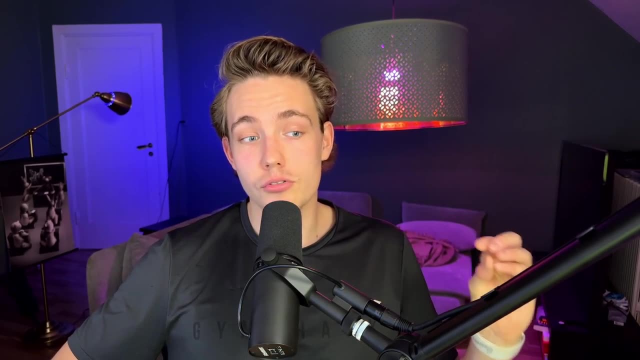 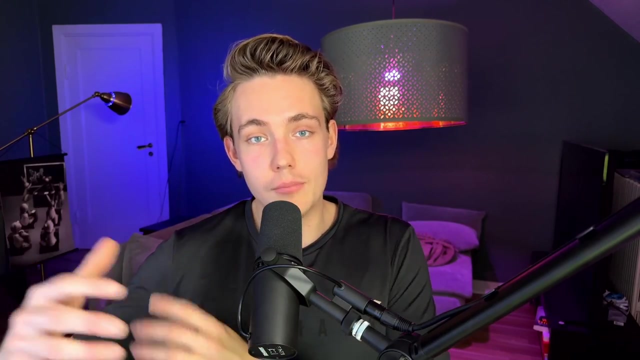 all the different kind of things and we also like put deep learning, optic detection and all those different kind of things on top of our computer vision foundation with the basic things and also the more intermediate things, with like, for example, like background subtraction, feature extraction. how can we actually like extract features and frames, match them to different kind of frames and then on? 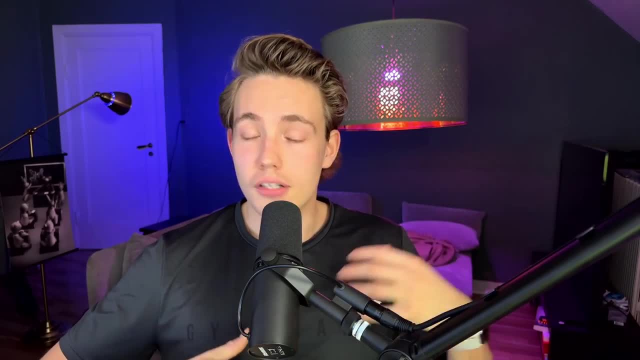 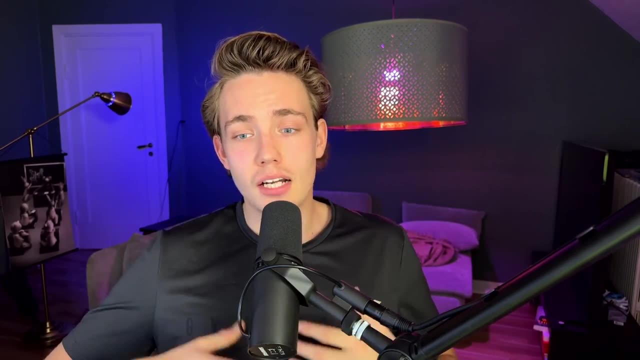 a more advanced level. how can we do like 3D image processing, depth estimation, how can we calculate depth with our images, and all those different kind of things with stereo vision? So this is basically like the roadmap. so start by learning the fundamentals of computer science. 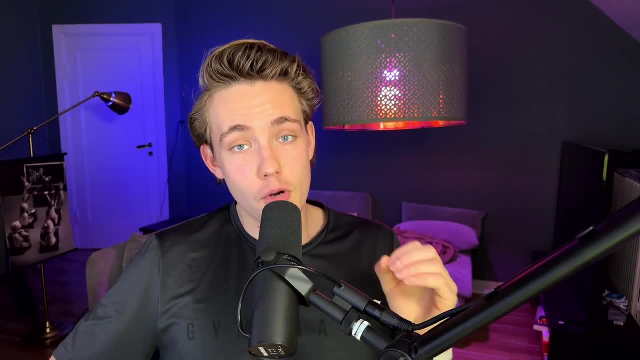 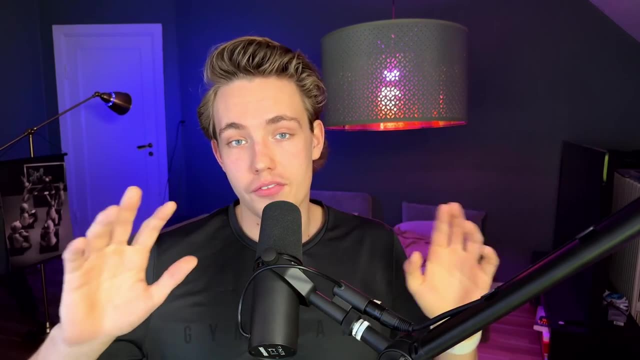 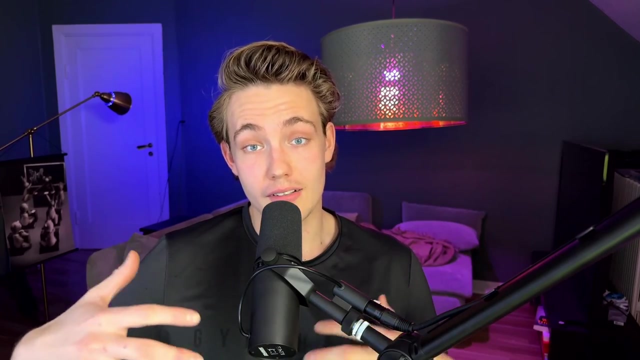 programming, including like data structures and algorithms, but, and the most important things, within math it acts. it's actually like algebra, linear algebra and calculus. you'll be able to use it for a lot of different kind of like computer vision applications when we're going to do some multiplication and all those different things, when we're going to act like do operations. 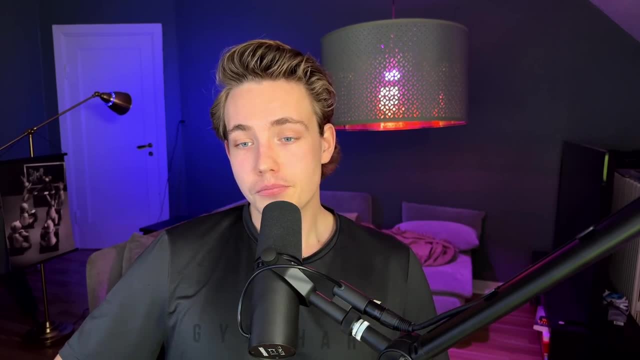 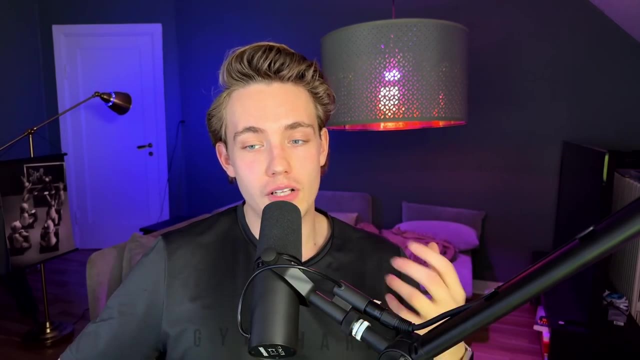 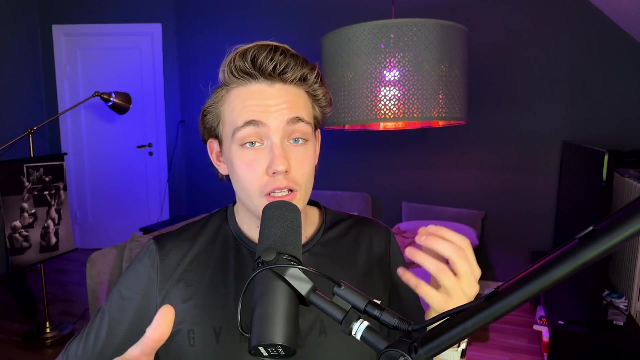 on images. we're basically just using linear algebra, then after that learn the basics of like image and video processing, including, like these different kind of techniques for like, like transforming and actually like just analyzing visual data. we're doing a lot of different kind like transformations, filtering methods and all those different kind of things. 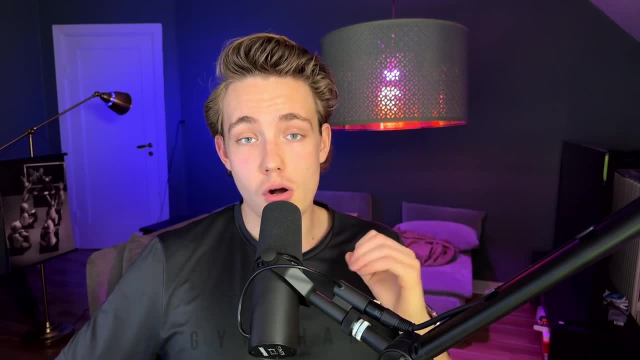 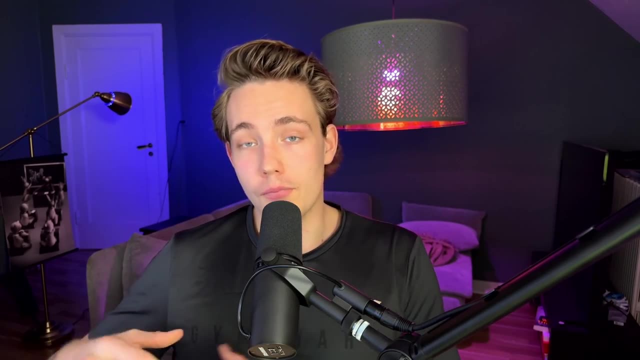 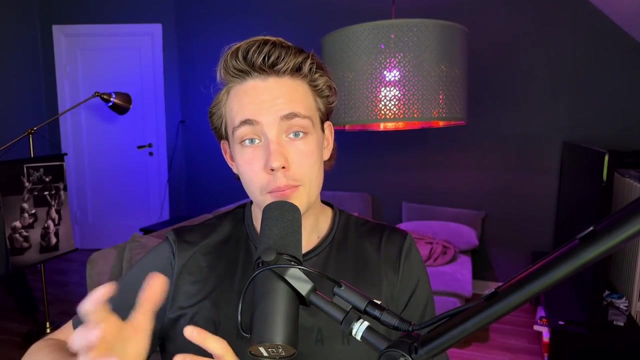 I both have like practical ways of how to actually do it, but I also go over the theory of how these algorithm filters and transformations act like works on the math level as well. when you know all those basic things, you can actually just take it into another step. so those are the more like. 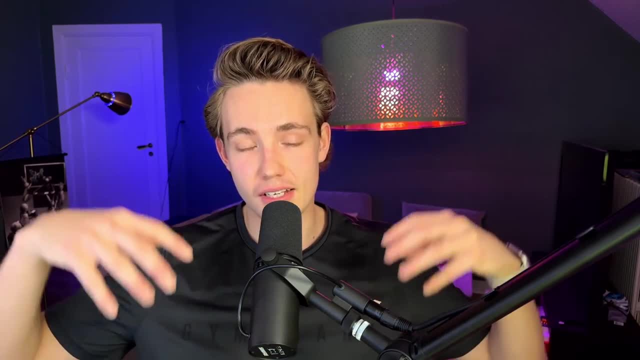 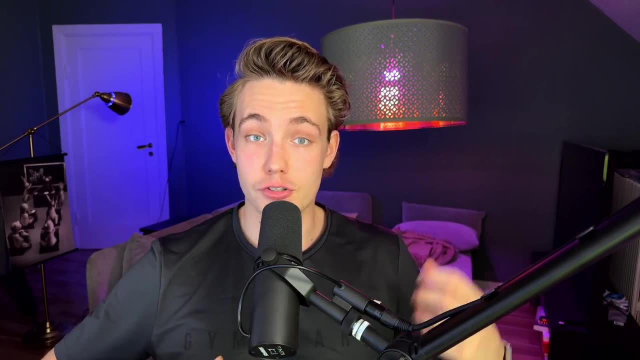 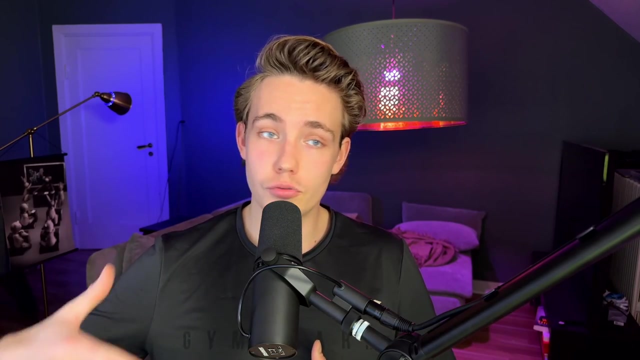 basic steps for actually getting into computer vision. now we can take it to an intermediate level where we actually go inside like feature extraction, processing and identifying and extracting information from our images. so basically we're just giving some images and then we actually want to do something with it. we want to be able to use it in real life because 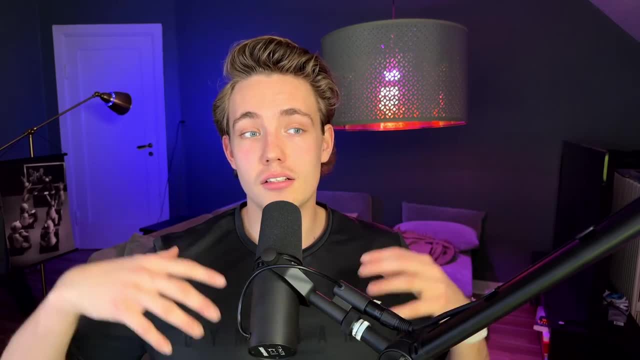 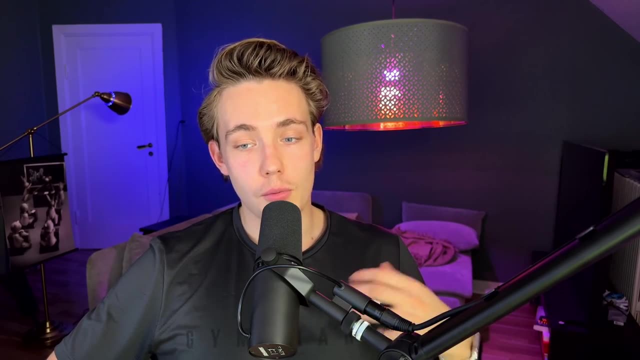 again like we're just learning computer vision to actually like get our computers to see something in the real world, so then we can take it to the intermediate steps, which is actually like feature extraction. we want to like do, for example, like it's detection, color histograms. how can I actually 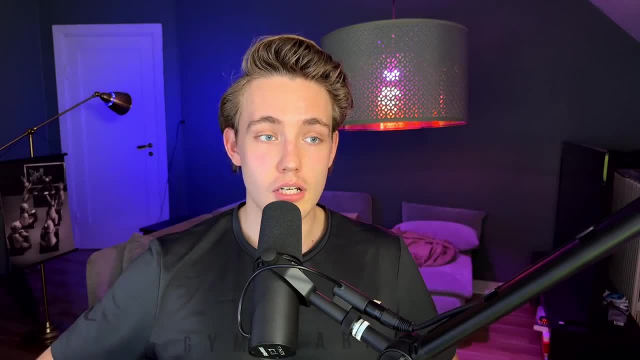 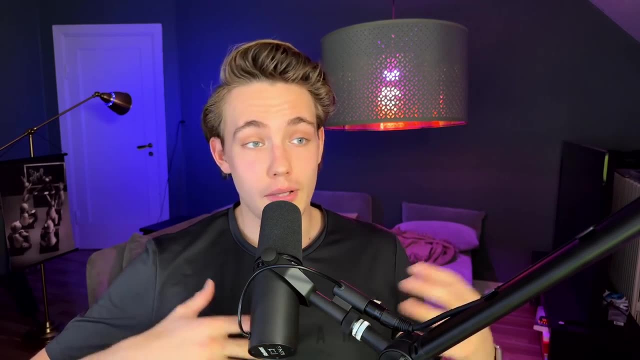 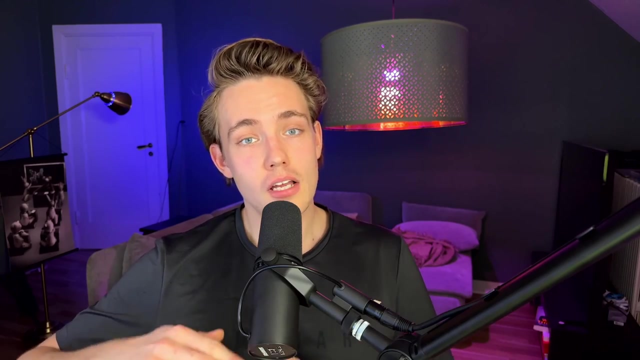 get information from color histograms? how can we manipulate our images so we can actually like see more information in our images without doing anything else than some post processing, playing around with some histograms and so on? and then again we can just add like pattern recognition, optic detection and all those different things, which is basically like on a bit more high level. 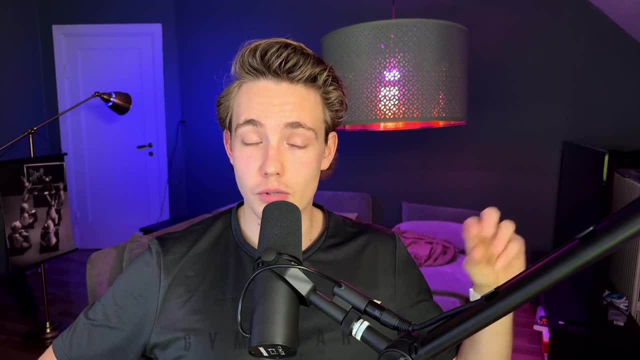 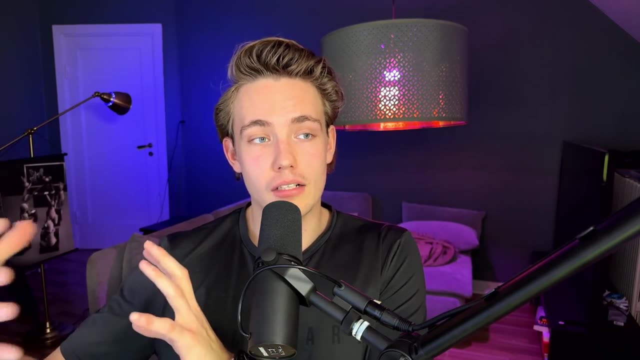 so when we have the basics, basic operations of computer vision, we have the basics. then we go to the media step, extract features and all those different things, and then the next level is basically just combining the intermediate steps and the basic steps. we go up on an even higher 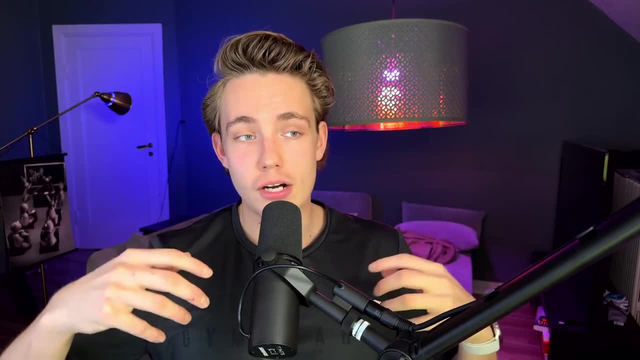 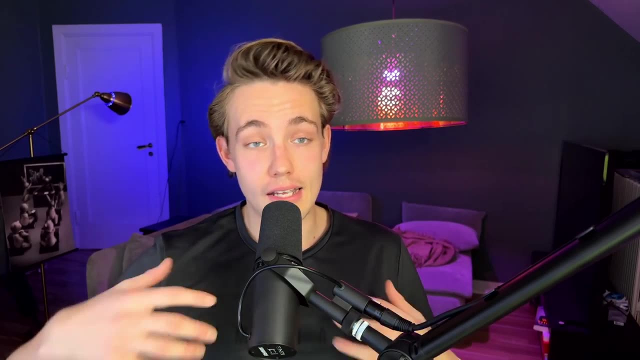 level. we combine all those different things. we do feature extracting to try to like find a 3D information in our images. we do stereo vision, optical flow, optic detection and then, when we actually get to that stage, we can try to like get into deep learning. how can we combine deep learning? 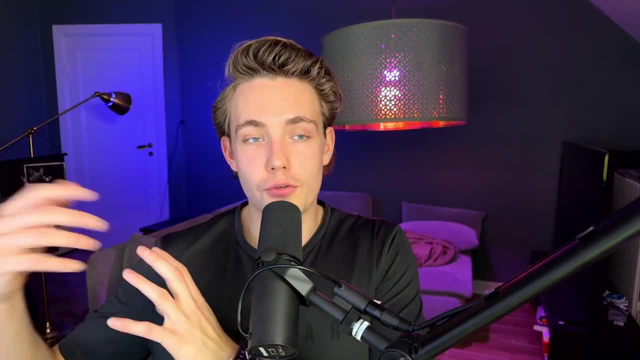 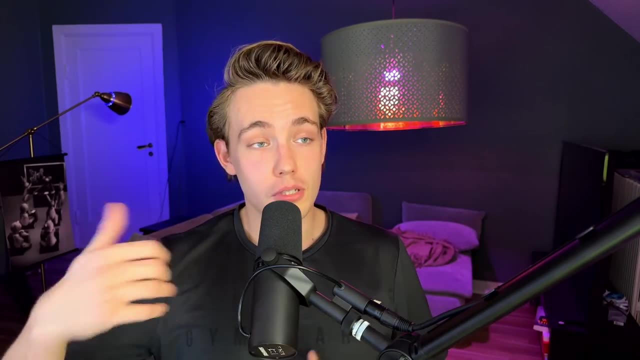 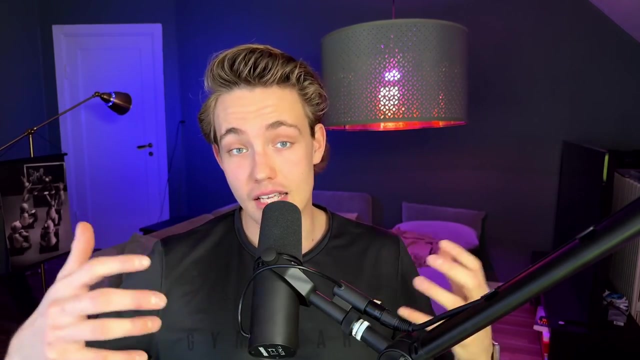 with computer vision because actually you can just take your images, throw them through some deep learning models. you can then do optic detection, optic segmentation and all those different things. but the more advanced computer vision stuff is actually like 3D reconstruction, understanding, understanding just seeing you're in and understanding what you actually see in the 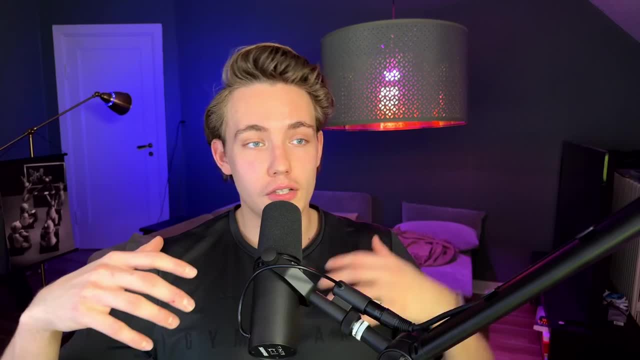 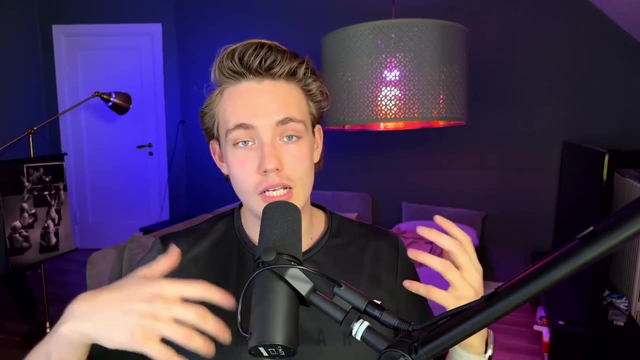 images and then also visual tracking. so again you can both like do detection in your images. so let's say we want to do like a person detector, then we can actually just detect that person walking around in the image frame. but sometimes you might lose track and we actually need to actually track the. 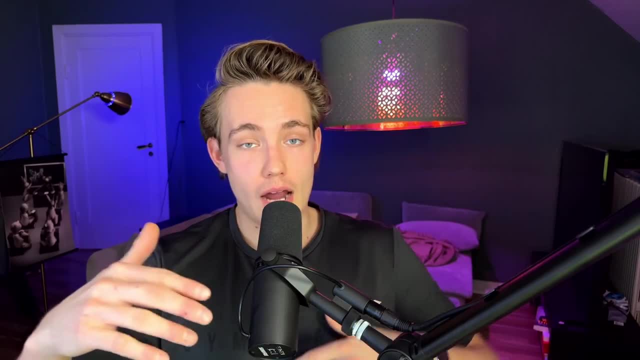 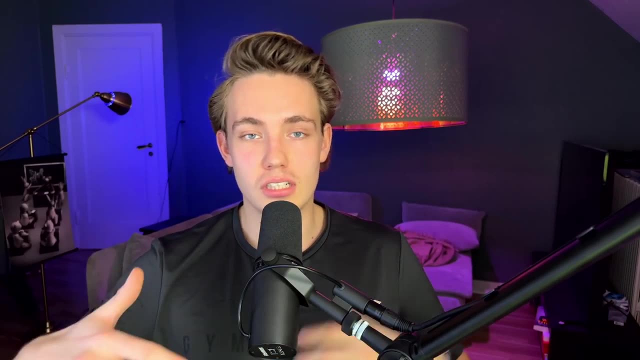 exact optics moving in the frame, then we can also add another step. then we're adding tracking on top of our detections and now we actually get to a really advanced level. and when we're at that level within computer vision and deep learning we can actually start to make some really useful things. 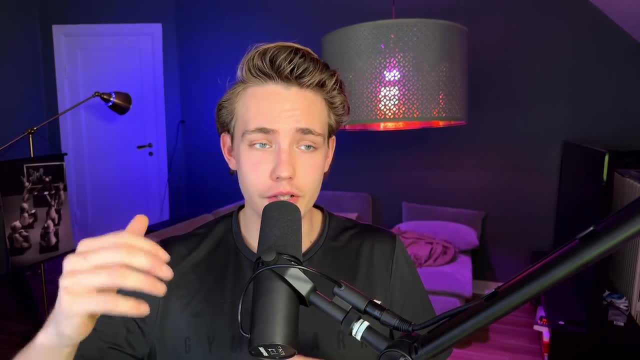 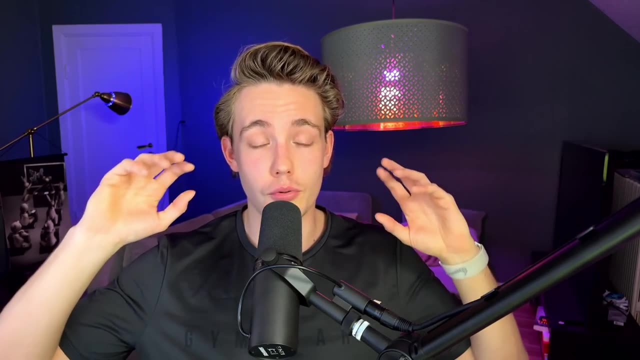 for the real world and then when you're at that point, you're really really good at computer vision. you can do a lot of different things. you can actually work with different like projects, concepts. you can do like pretty much everything within computer vision. of course, new things come. 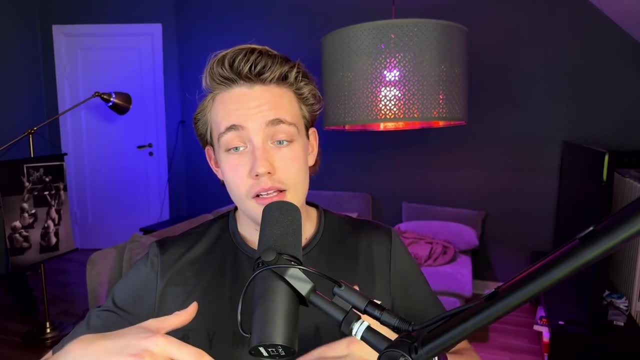 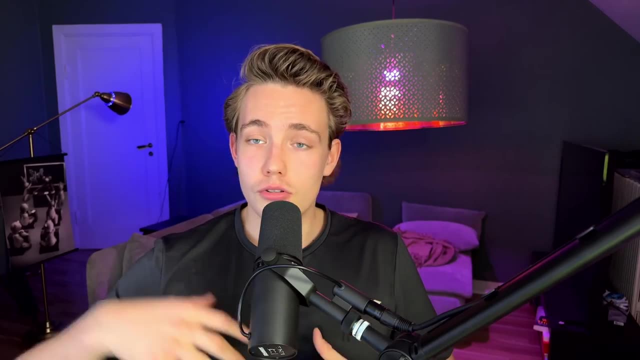 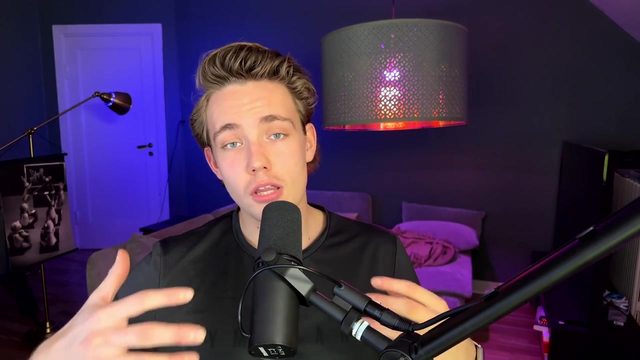 out all the time. you need to keep keep updated with that again as you continue to learn and do computer vision also like. participate in different kind of like online communities, also here in the channel. be active on the channel in different communities. learn from other people. like talk to other people also. if you teach other people the concepts and the ideas that you learn. 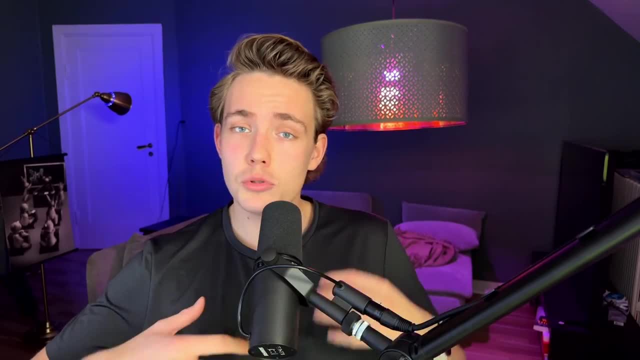 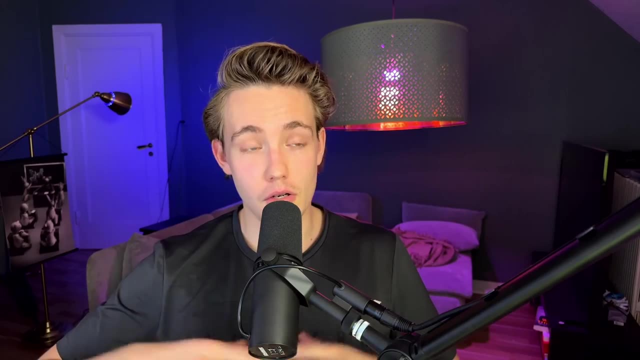 by yourself, then you will actually like understand them way better. this was also actually like one of the main reasons I started this YouTube channel was to actually teach you guys something about like computer vision, deep learning on all those different things, and just as the time went by, I 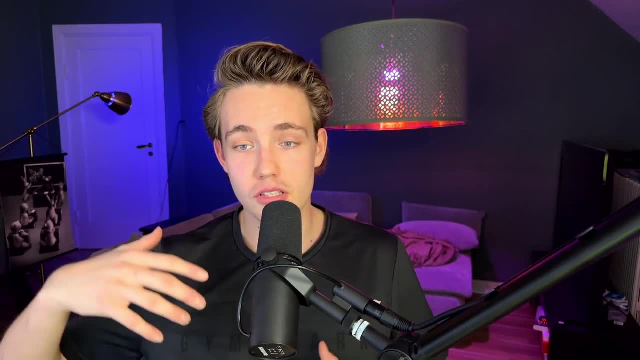 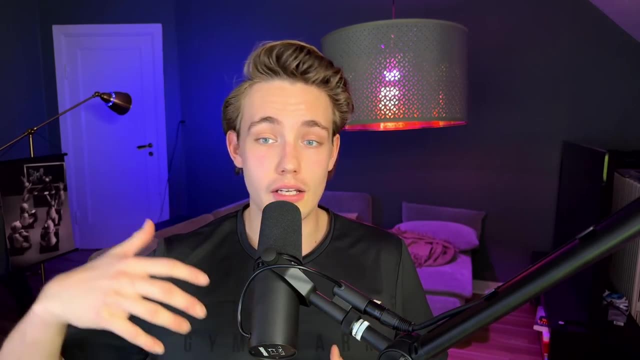 just get got way better at computer vision, all these different things. by just like talking about them, teaching them to do, you guys, I just gained a lot of more knowledge. um, I was actually like getting more into like implementing these things acts, like going from like theory to act, like implementations. how can we use this in the 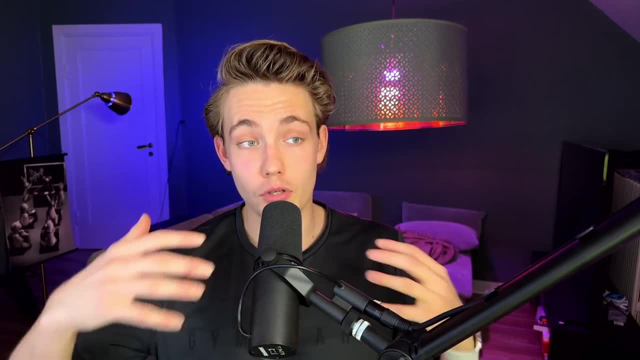 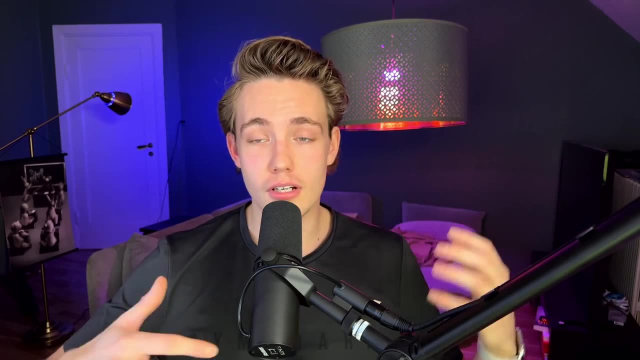 real world and then I just kept on improving, like my, my computer vision skills and and my understanding of computer vision and how it works. it just got way better by actually teaching, talking with other guys about it. um, trying it out again. if you want to be good at something, you just need. 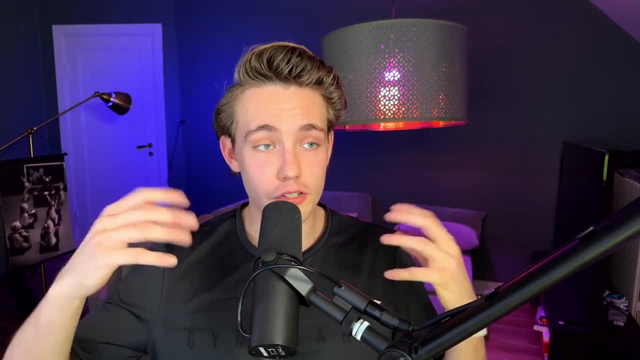 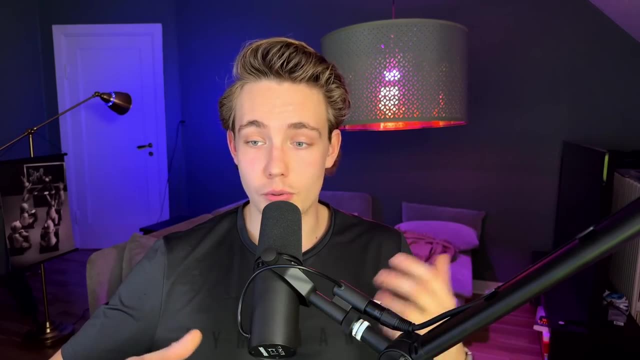 to do it in the hours. so my advice is basically just like participate, like talk to other guys, participate in different kind of like communities in forums, stay up to date like uh, get into like Twitter, like LinkedIn and all those different things. just stay up to date with the new things. 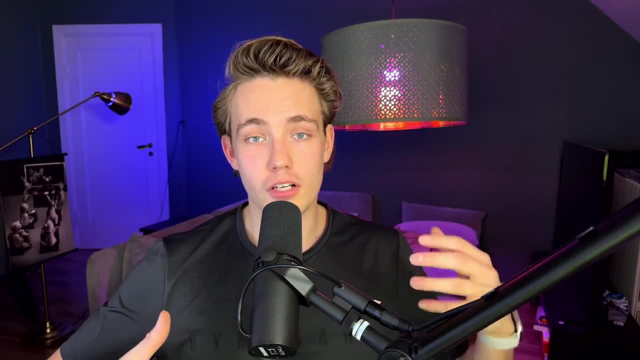 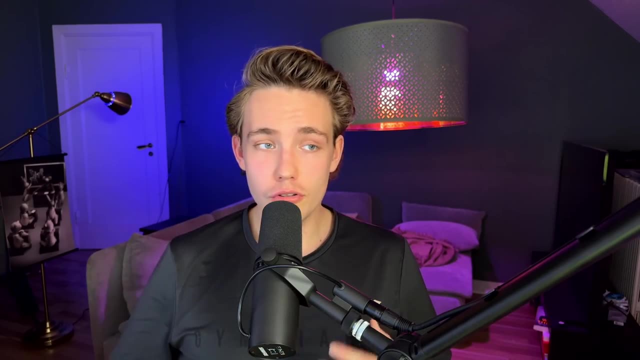 in computer vision once you have like the basic understanding on the fundamental levels or you're at the really high level, uh, you try to like do something useful with computer vision. you can also look at different kind of like conferences as all and all those different things. but 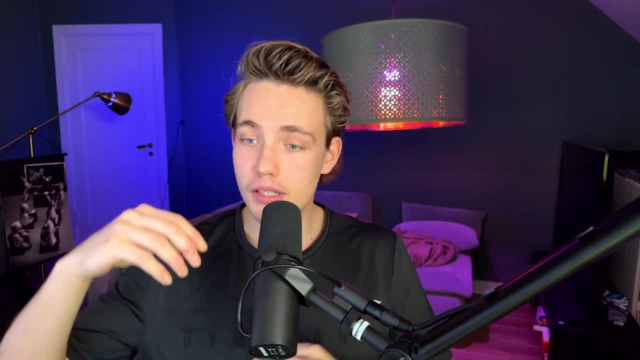 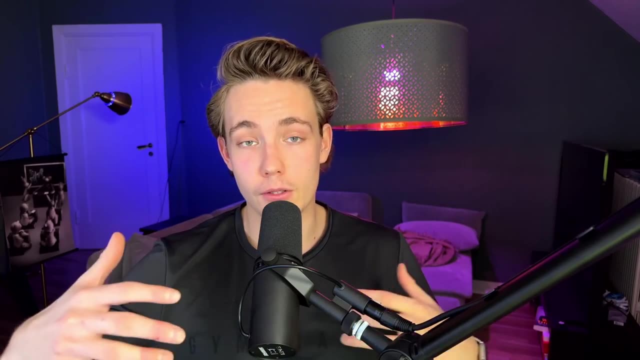 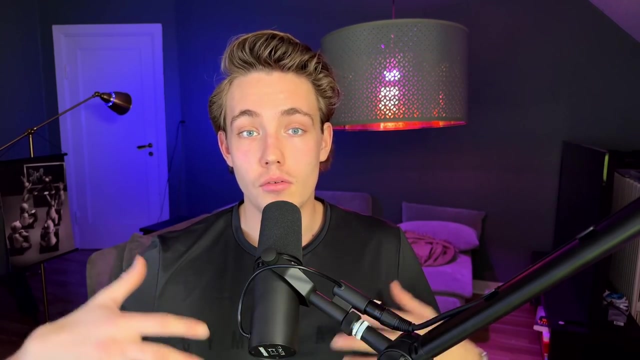 the most important thing is to actually just stay up to date, keep learning, and the way you learn is act like by implementing things. so, again, if you just like look at it at a fundamental and like theoretical view, you won't really be able to apply it, implement those different things in real world.